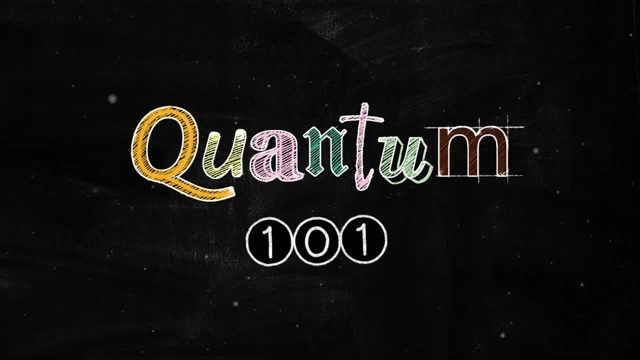 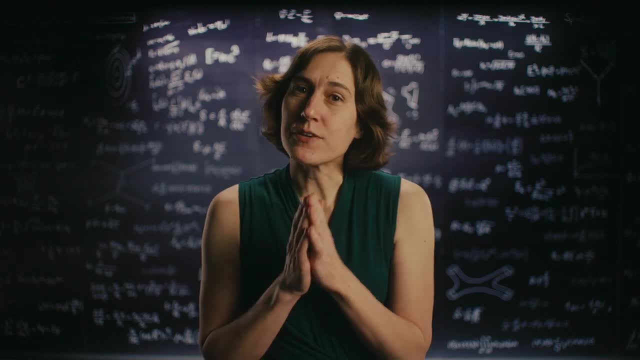 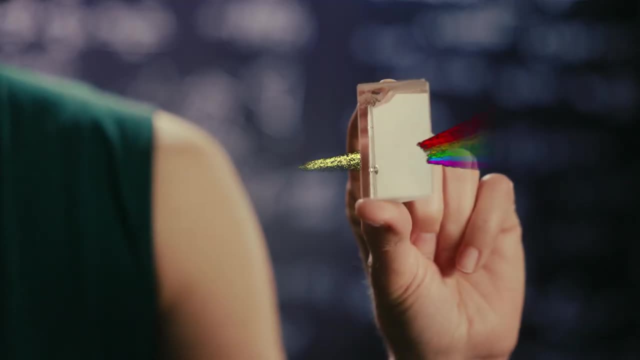 You may have heard that light can act like a particle and like a wave. It can bounce off a mirror like a particle and it can bend and spread out like a wave, For instance when it passes through a prism. With careful experiments we can see how light waves can interfere with each other. 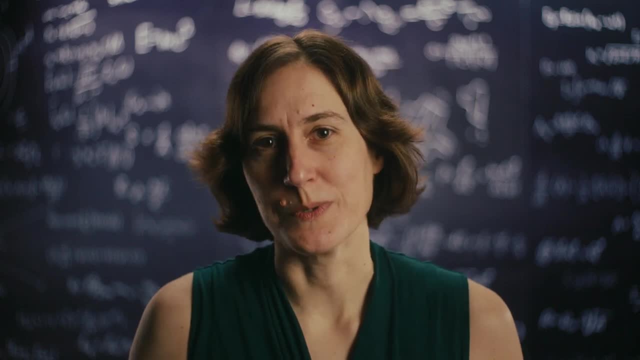 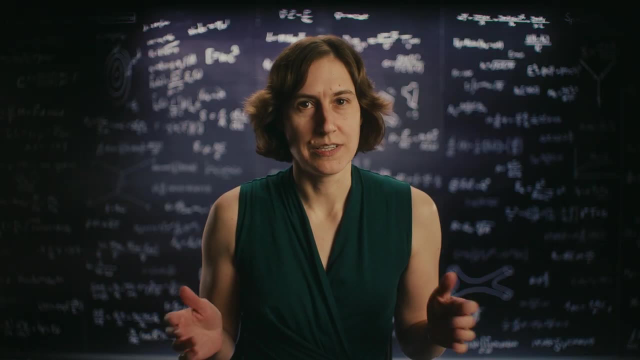 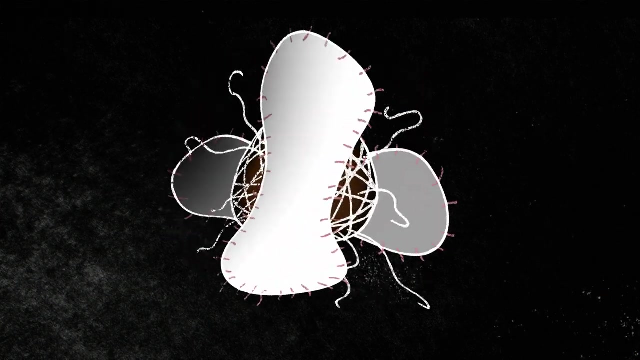 But did you know that particles can act as waves too? This is one of the central ideas in quantum mechanics. Everything has a wave nature: Light particles and even, in an unobservable way, macroscopic objects like baseballs and people. One way to see the wave nature of light is through 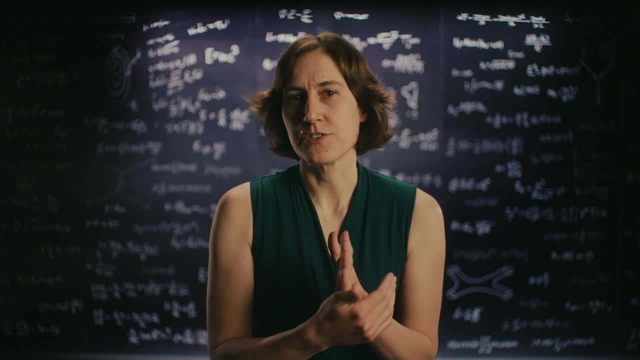 diffraction: the way that light bends around the sharp edges of objects or creates patterns when passing through narrow gaps. In the dead of night, light can be seen as a wave but not as a particle. In the dead of night, light can be seen as a particle, but not as a particle In the dead of. 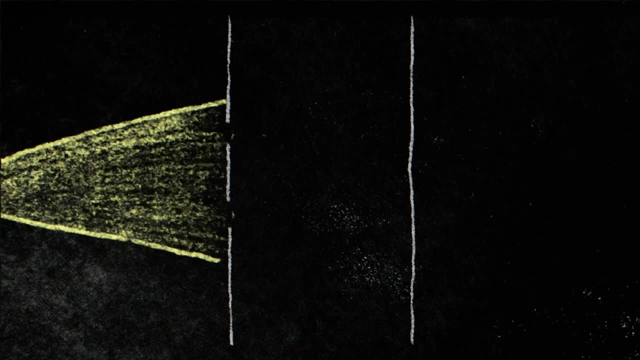 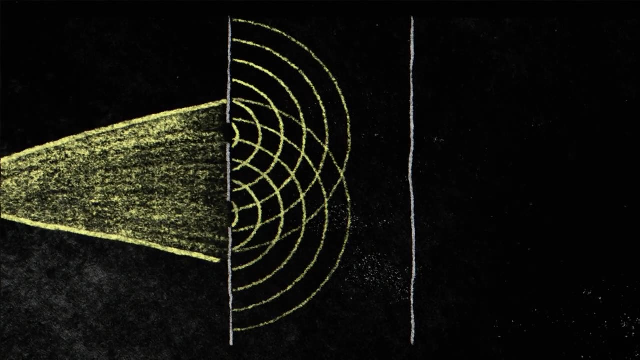 night. light can be seen as a particle, but not as a particle In a double-slit experiment. laser light passes through two slits in a wall and spreads out like a wave. as it passes through, The waves coming from each slit interfere with each other, creating a pattern of light and dark. 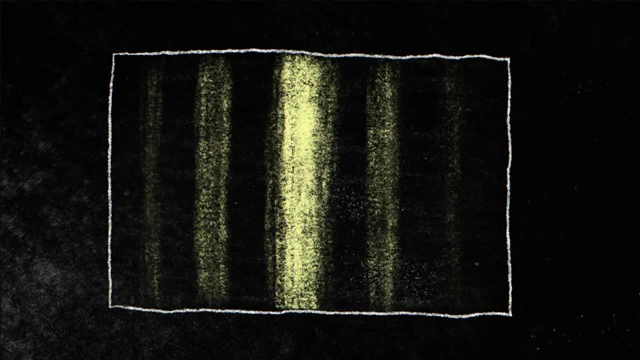 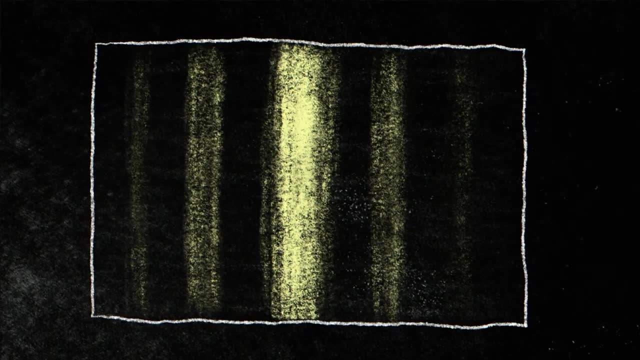 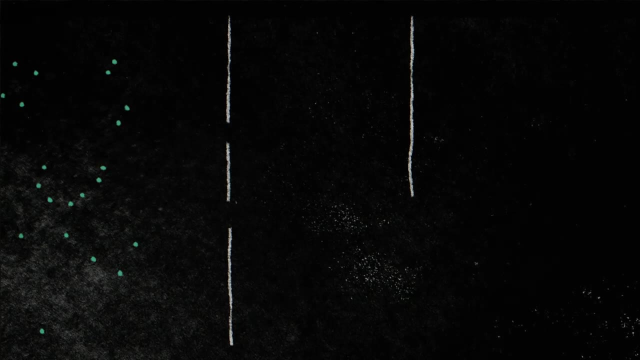 spots on a wall on the other side. This happens because when two crests or two troughs of a wave meet, they add together, but when a crest and a trough meet, they cancel out. But what if, instead of laser light, you throw particles at the wall? 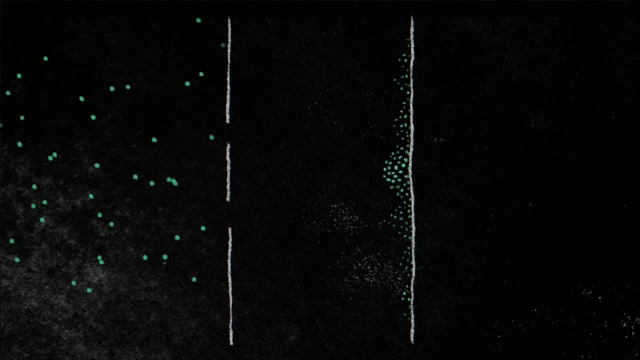 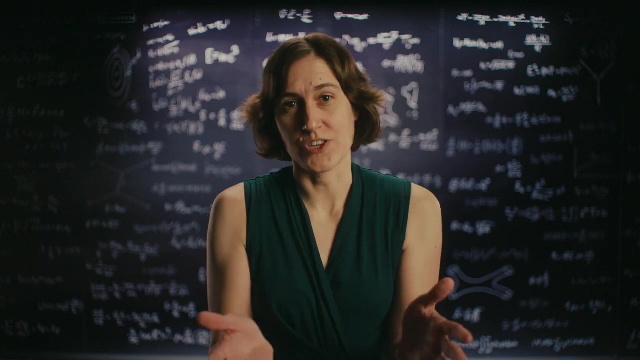 If you have a powerful electron beam, you can see that instead of two spots directly behind the slits or randomly distributed spots, an interference pattern will appear. just like with the light, The electrons are behaving like waves and interfering with each other. 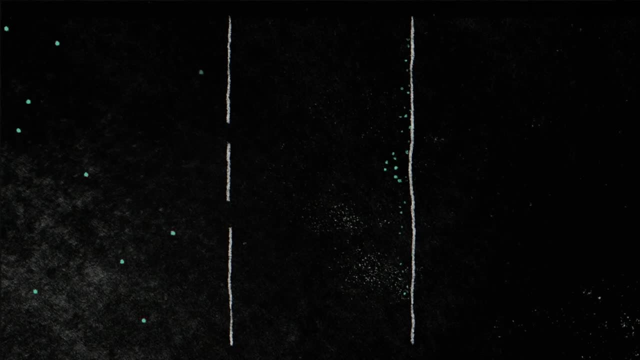 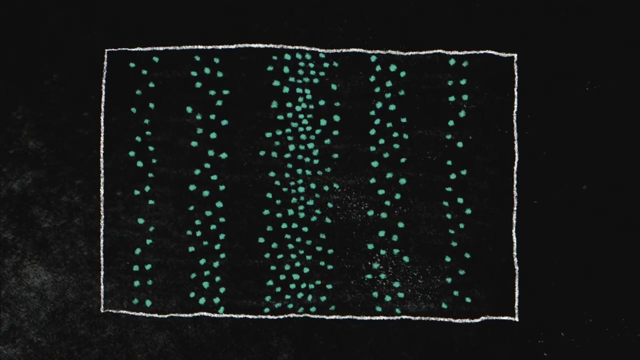 Even weirder. you can slow the experiment down and send one electron at a time. Each electron will pass through and hit the wall at a single point, But over time you'll see that the same interference pattern appears even though no other electrons were passing through at the time, to create interference. 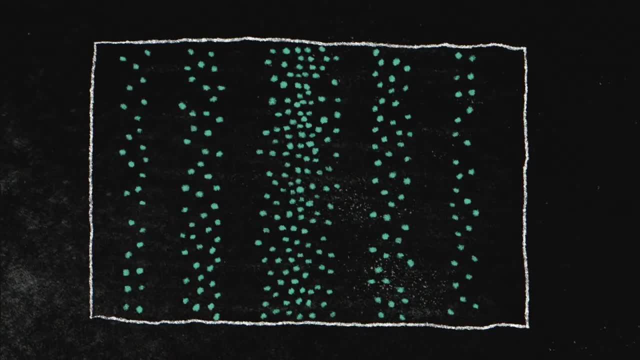 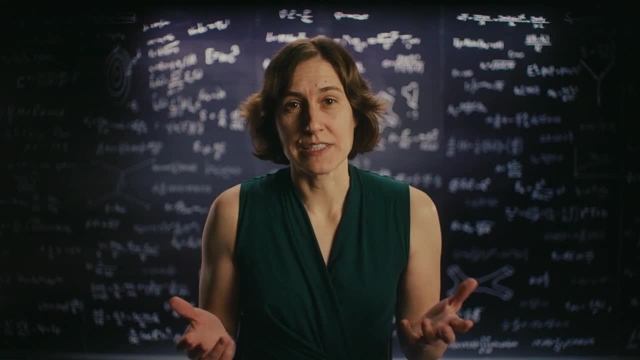 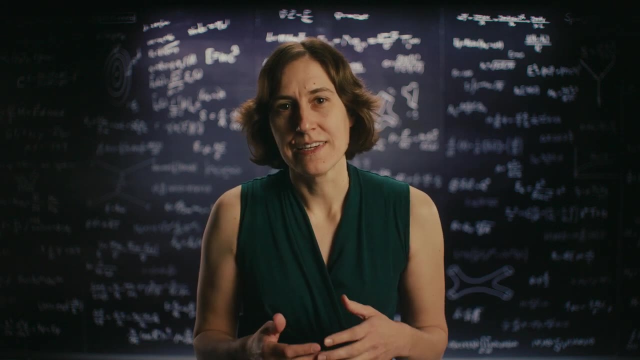 Apparently, each electron is actually interfering with itself. This is the crux of wave-particle duality. Even something we think of as an individual object, like an electron, has an essential wave-like nature and acts as a wave when it's moving through space.